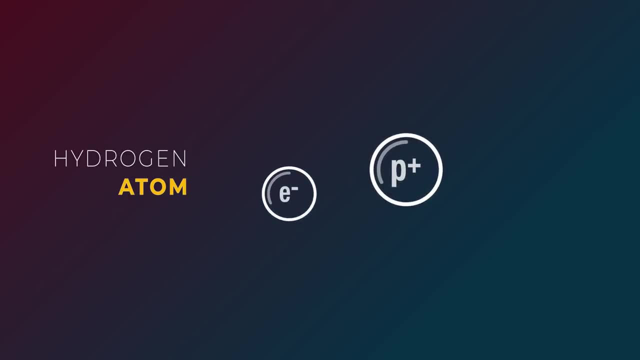 made of a proton and an electron, and these are the protons that we're eventually going to be accelerating. We take a piece of pure molybdenum about the size of a teabag and use it as a source of extra electrons. We run electricity through it and we end up with 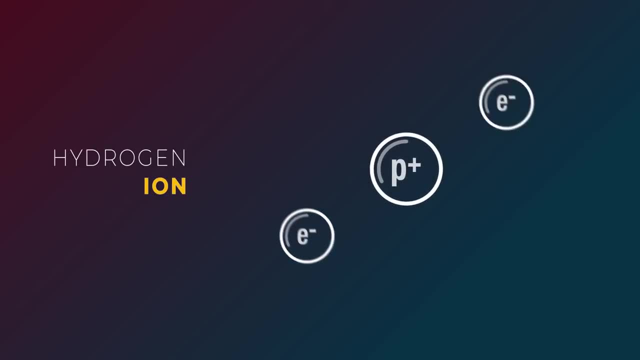 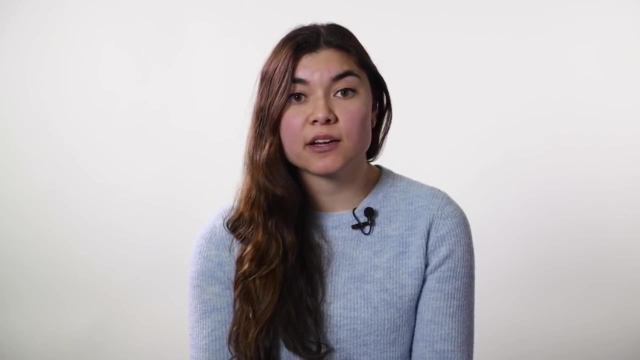 a gas of hydrogen. ions that each have an extra electron Because they're charged. we can manipulate these ions with our magnets. We can use an extractor to pull these ions in the right direction, which starts the beam. The first stop is the RFQ, which can bunch. 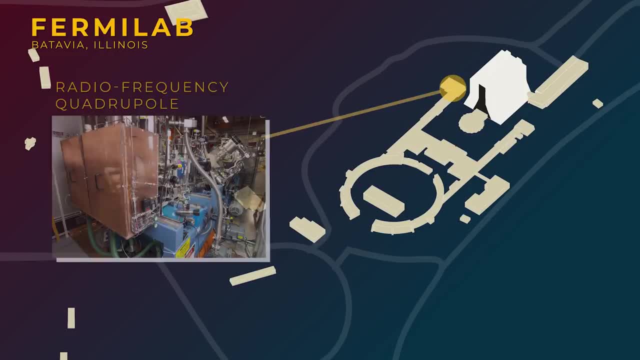 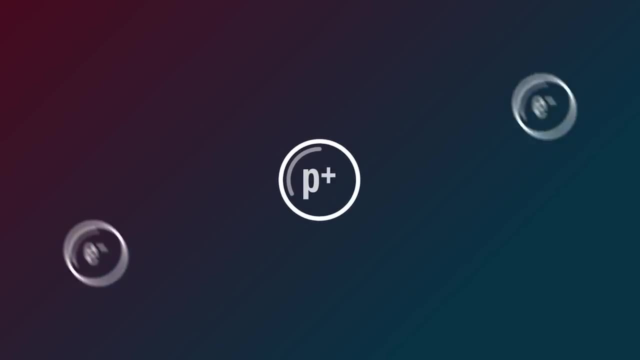 out some of these ions which can start to raise the beam but then start to get smaller together and speed up the ions. It hands them off to the linear accelerator or LINAC, which gives them even more energy. At the end, these extra electrons are stripped off of these ions making. 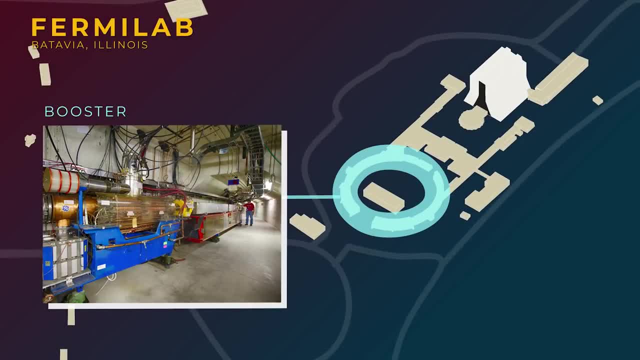 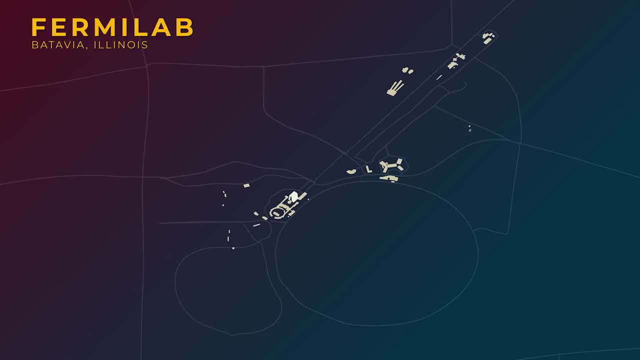 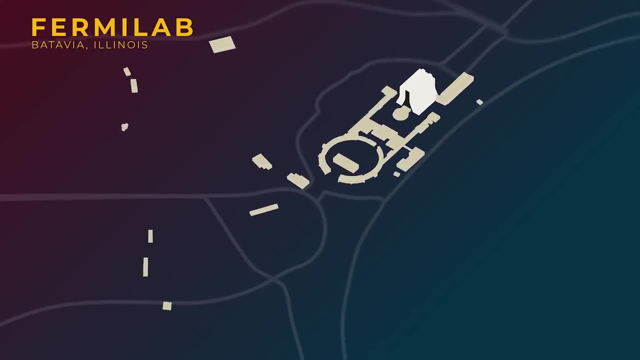 our proton beam. Then it gets handed off to the next accelerator, the booster. The protons can take different paths to experiments around the site, including to the test beam facility, muon experiments and neutrino experiments. Fermilab is unique because we can make neutrino beams at 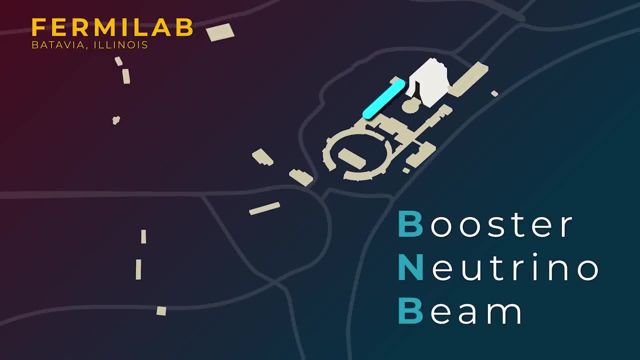 two different energies. For lower energy neutrinos we use protons that come straight out of the booster. This booster neutrino beam makes neutrinos for the three experiments in fermilab's short baseline neutrino programme and the anrainexperiment. For higher energy neutrinos. 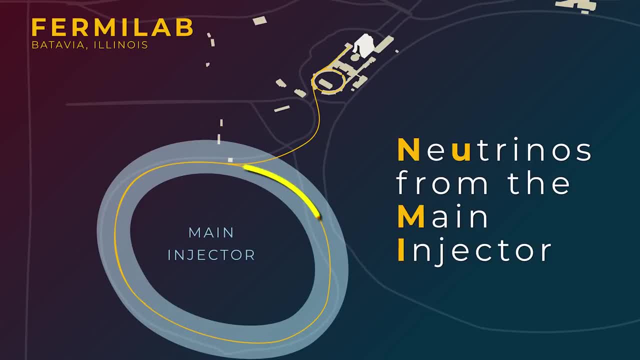 operators can move the proton beam into an even bigger accelerator. the main injector, The noumie beam, is what we use to form the production of the neutrinos used for the Minerva and Minos experiments and now used for Nova. The main injector will also be used to make neutrinos for Dune, But either way it's a. 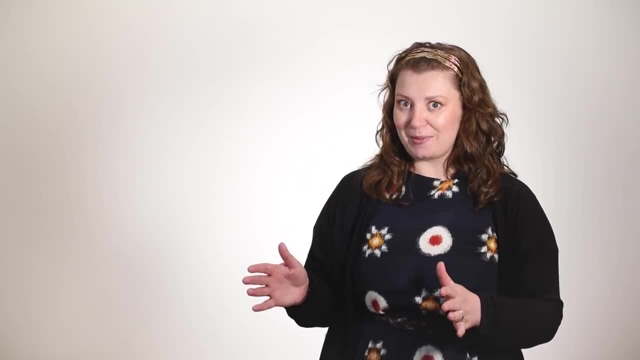 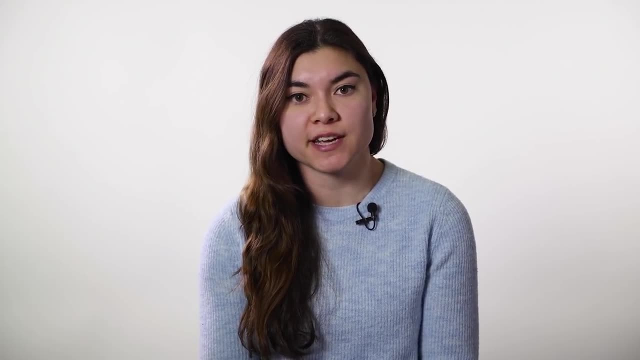 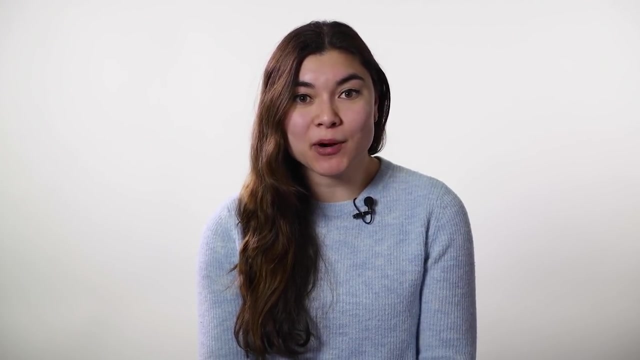 similar process to go from proton beam to neutrino beam. That's right. we use the magnets to steer the protons in the right direction, so they're traveling toward a neutrino detector, which can be anywhere from several hundred feet to several hundred miles away. Then we get to do the cliche particle physics thing. 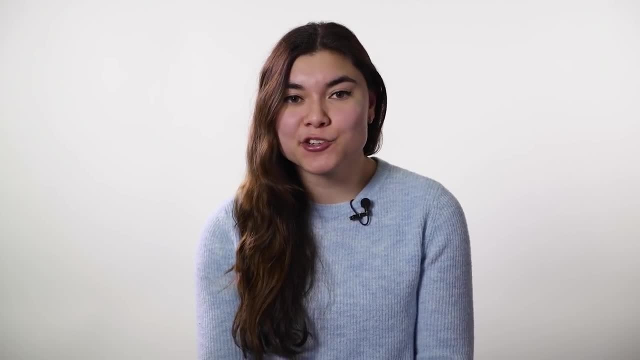 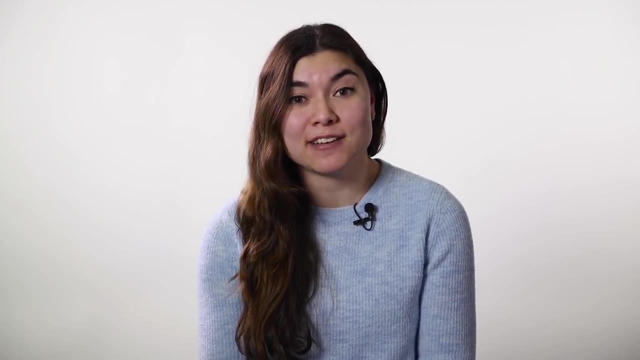 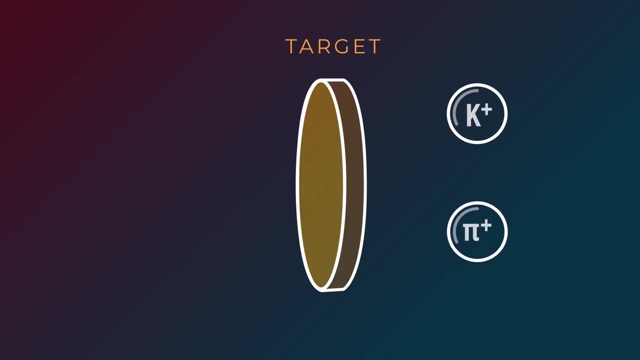 and smash them. We have different options for these stationary targets, like solid graphite or beryllium, and these targets have a tough existence. They're absorbing a lot of energy from the protons. When the protons collide with the target, it causes this spray of energetic new particles. This includes 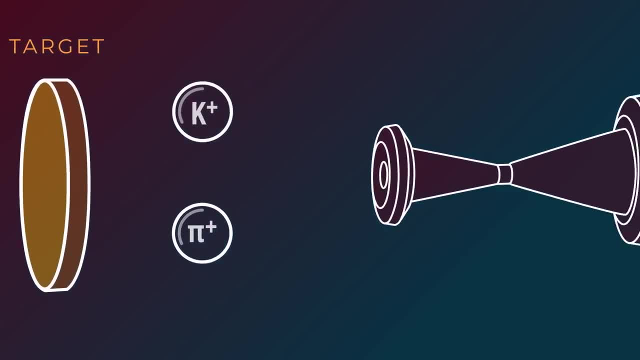 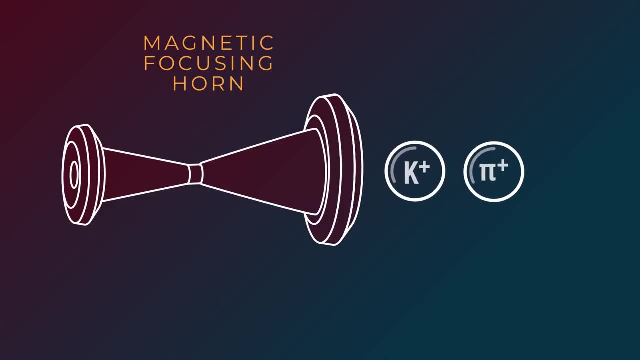 some charged particles called pions and kaons, which we can steer using more magnets. They travel through things called neutrino horns or magnetic focusing horns. These are essentially big magnetic focusing horns. These are essentially big magnetic focusing horns. These are essentially big magnetic funnels that get the particles condensed back. 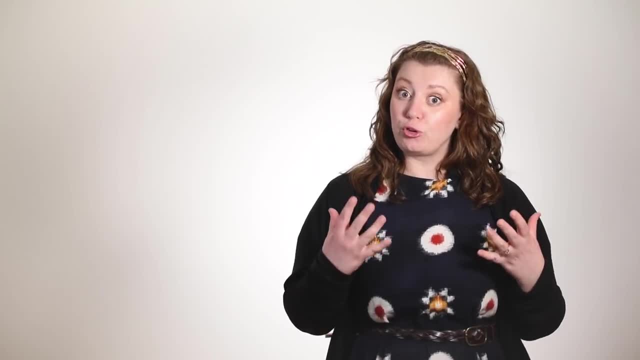 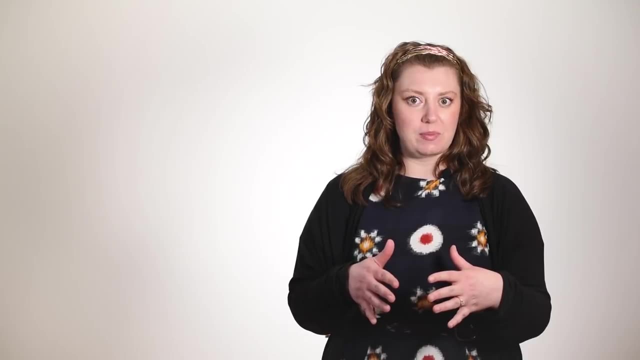 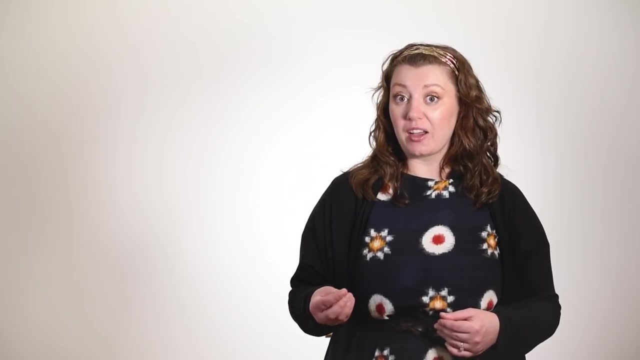 into a narrow beam. To make a beam of neutrinos, we set the magnetic field in the horn so that it focuses positively charged particles towards where we want the neutrino beam to go and defocuses negatively charged particles. As our charged pions and kaons fly away from the target, they decay, producing neutrinos. For example, a positively charged pion will decay to a positively charged muon and a muon neutrino. We can also reverse the field in the magnetic horn and make a beam of anti neutrinos. and yes, it does feel very cool to say we can make a beam. 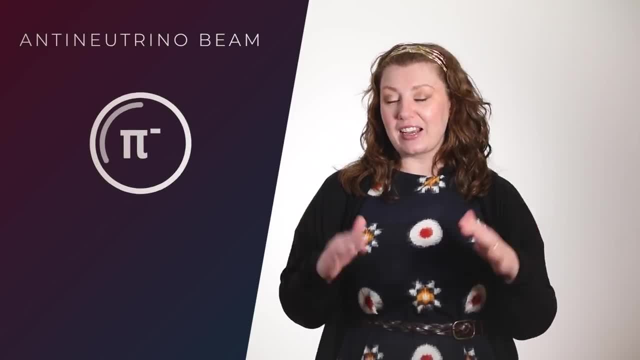 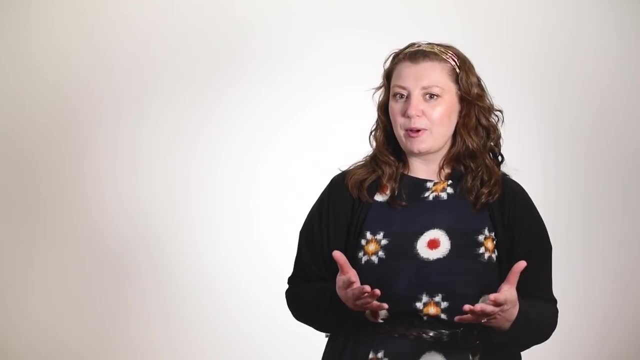 of antimatter To do that. we focus the negative pions and wait for them to decay into a negative muon and a muon anti neutrino- Neutrino experiments regularly run in both neutrino and anti neutrino mode, and that is one of the ways we can. 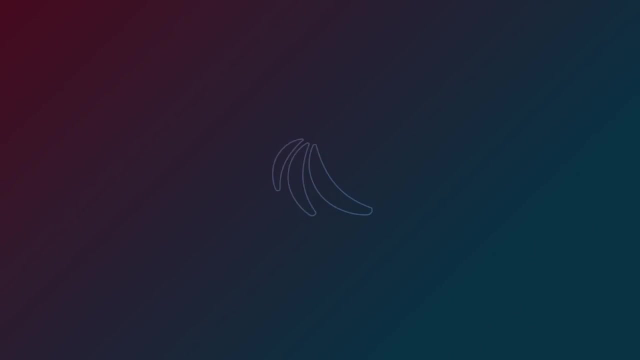 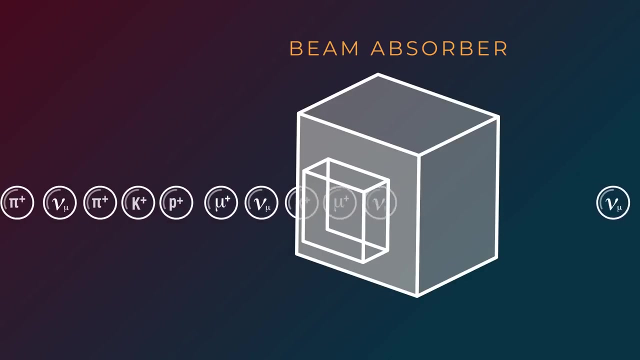 study how matter compares to antimatter. The last step to making a neutrino beam is stopping all of the particles that aren't neutrinos. We put a material like concrete or steel in the beam path and this absorbs the muons, pions or kaons that haven't decayed yet and any. 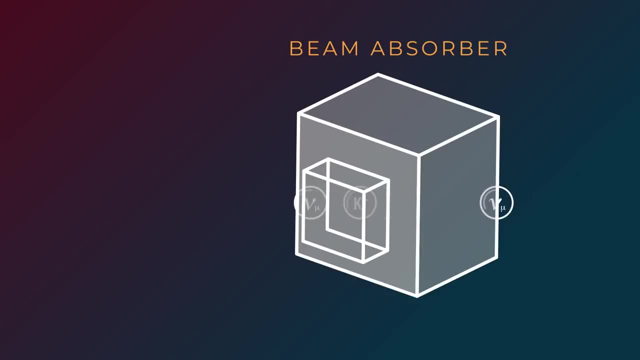 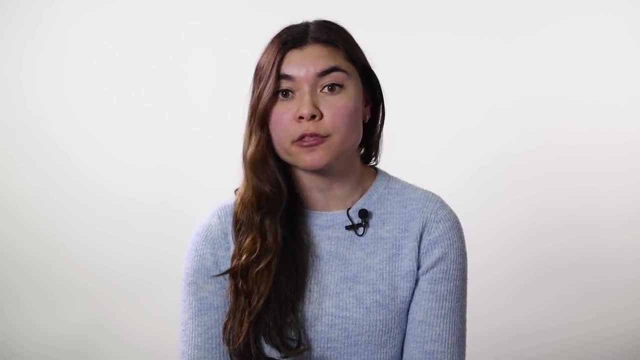 stubborn protons that have made it that, far After they're produced, the neutrinos are on their own. We, as operators, can no longer control their flight path. The neutrinos travel straight through whatever is in front of them, eventually arriving at the detector. This whole process. 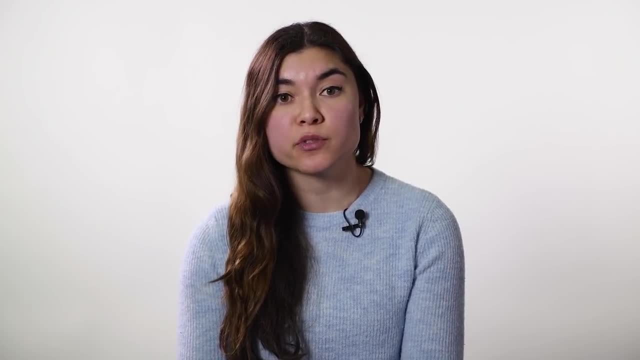 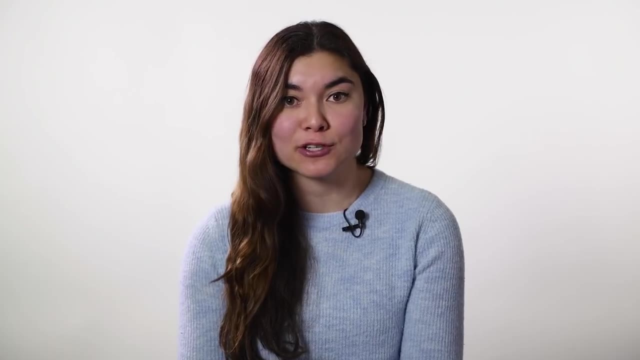 happens really quickly. We're able to send trillions of protons through the accelerator complex every second and produce trillions of neutrinos. You might be thinking: what does a neutrino beam consisting of trillions of neutrinos look like? And people always ask me: can you stand in the neutrino beam? Well, 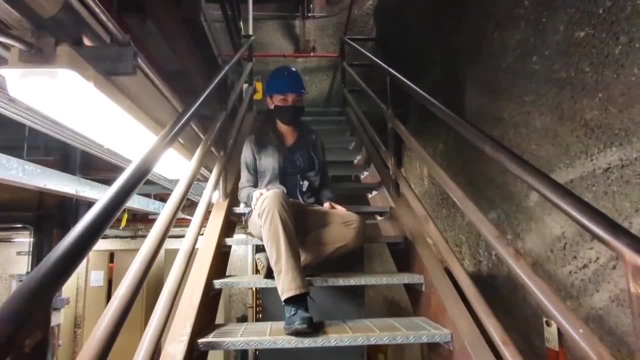 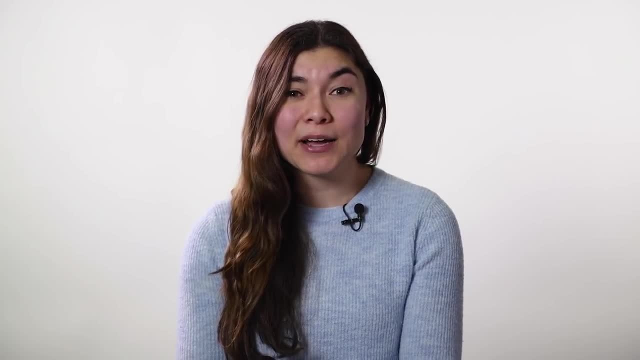 here's a video of me sitting in our underground experimental hall and you can see the white circle on the wall indicating the center of the invisible neutrino beam. I could sit there for about seven minutes before a neutrino would interact with me, and then I would be able to see the center of the invisible neutrino beam. I could sit there for about seven minutes before a neutrino would interact with me, and 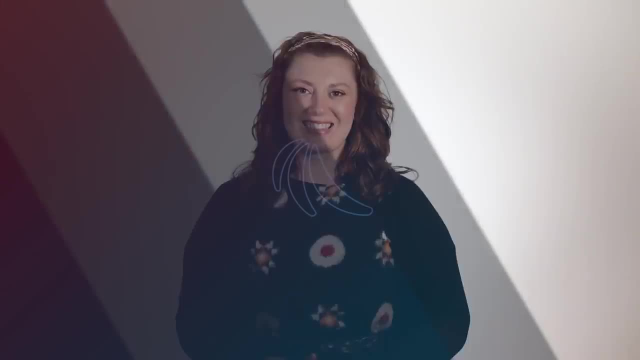 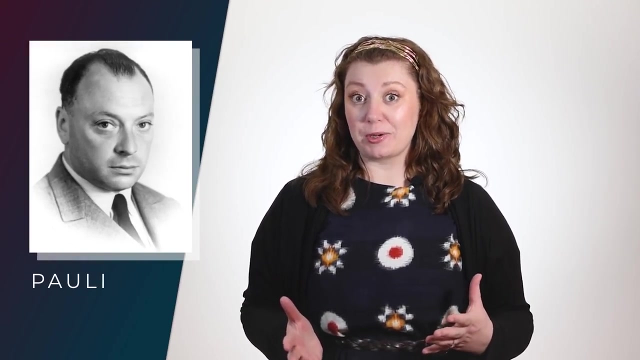 even if one did, I would never notice. Thanks, Laura. It's mind-boggling to think that in 1930 Wolfgang Pauli predicted neutrinos existed but thought we'd never be able to see them, And now we have the technology not just to see them but to.